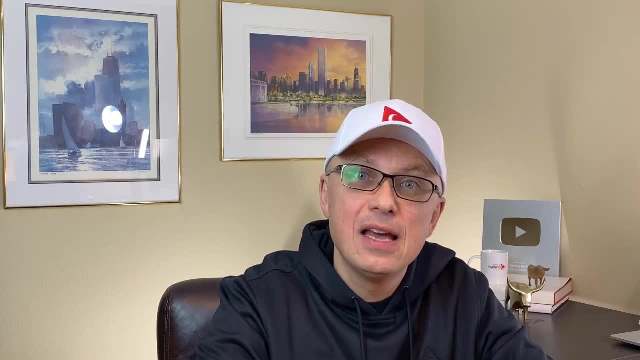 even though this is something you might consider doing as well. But if you see a different way of solving the challenge, please share it in comment sections so we all can learn, And also if you know other test questions that you'd like us to cover. 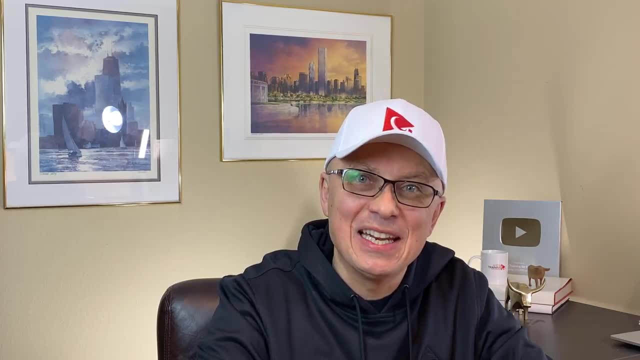 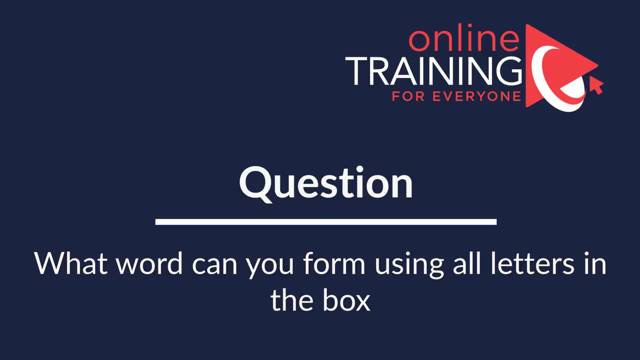 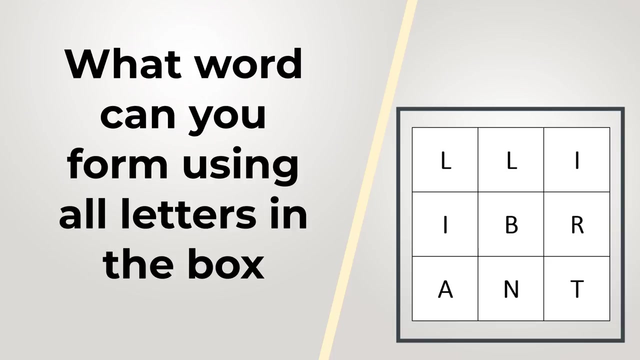 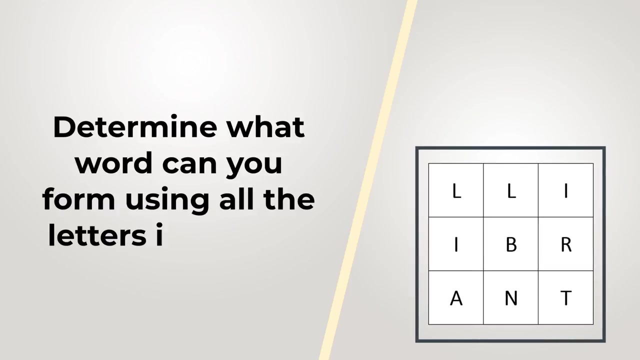 in the future videos, please share them in comments. Let's go ahead and get started. If you like solving word puzzles, this question might be for you. You need to look at the nine letters on the left and determine what word can you form using all the letters in the box. 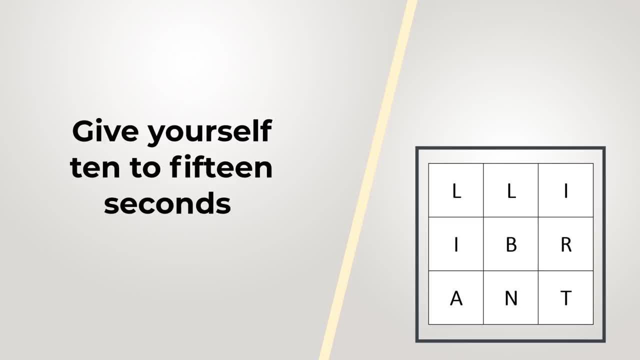 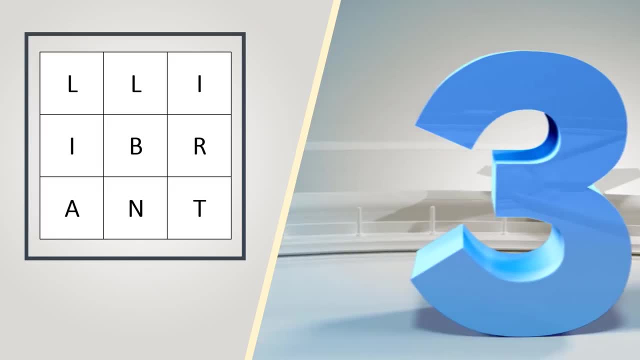 Give yourself 10 to 15 seconds and see what's the most important question, The best way to solve the problem. I'm going to give you a quick hint. Sometimes, as I move from left to right, or from right to left, or diagonally, or up and down, you might get an idea of what kind 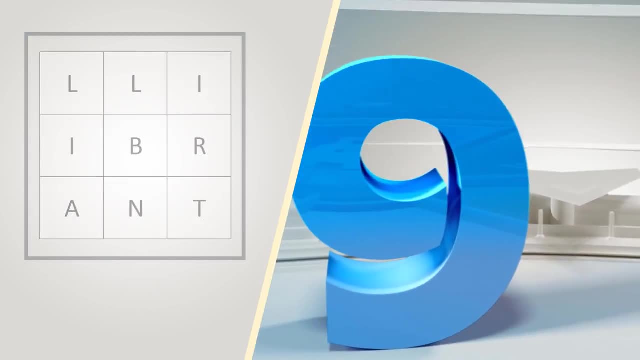 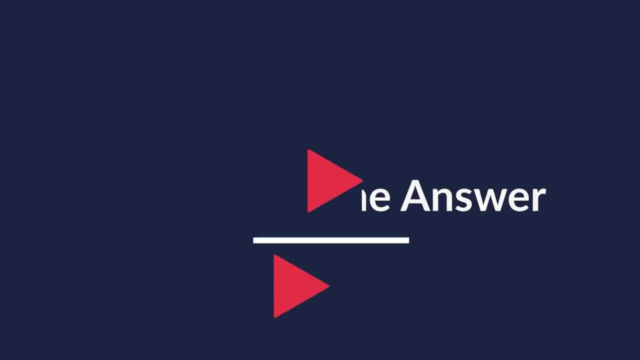 of word you can form, So hopefully this tip will help you here. Do you recognize the pattern? Let's continue to see how we can solve this challenge and get to the correct solution together. Obviously, there are many words that can be formed with the letters in these nine boxes. 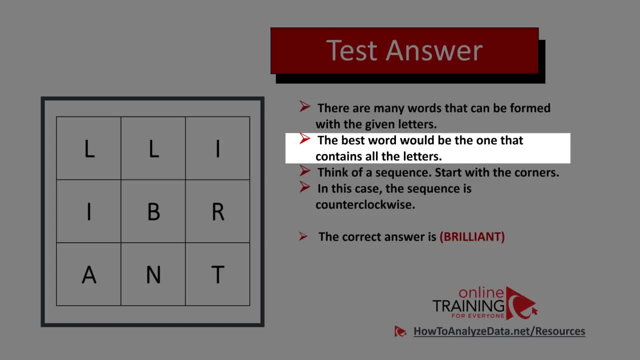 But the best word that we can form is the one that we can use to solve the problem. It contains all the letters and contains no duplicates. If we think of the sequence and start in the middle and then go around counterclockwise, we see that we can form. 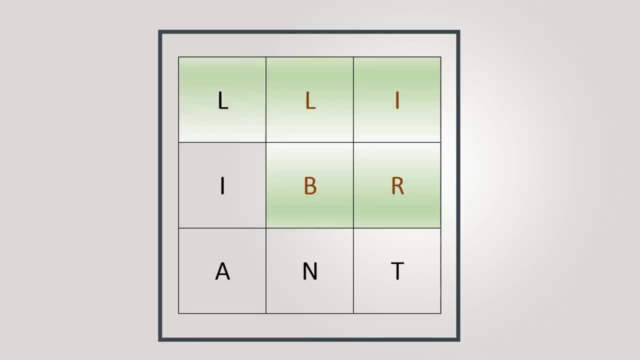 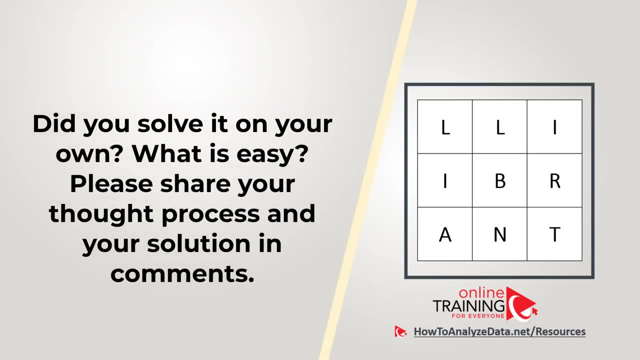 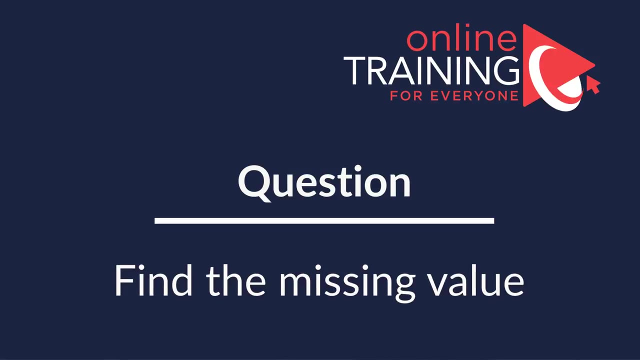 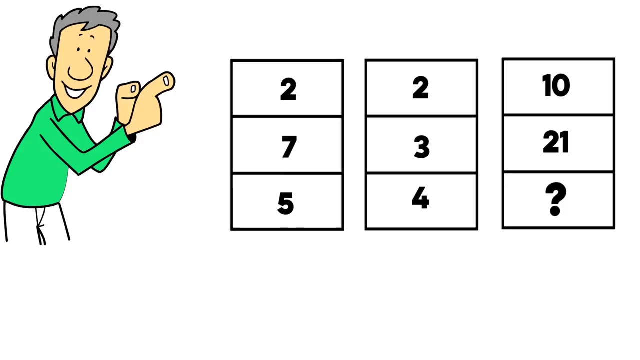 a word brilliant, So the correct answer is brilliant. Hopefully you've nailed this question and got to the correct answer on your own. I'm extremely excited to share with you the question that tests your pattern recognition. You need to find the missing value, which is highlighted by question mark. 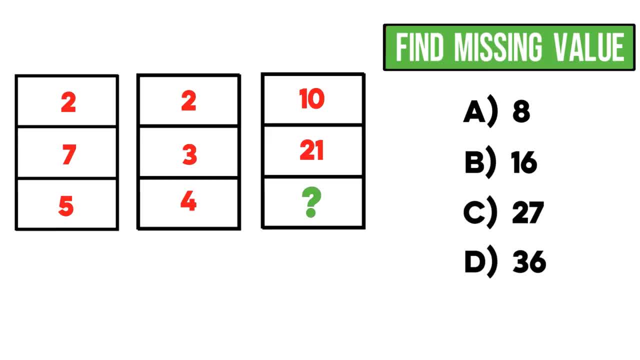 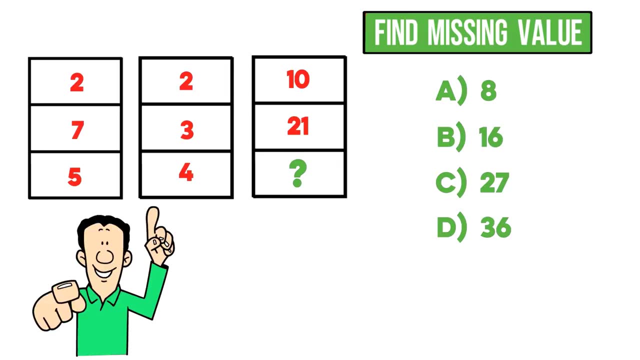 And you have four choices to choose from: Choice A: 8. Choice B: 16. Choice C: 27. And choice D: 36. Do you think you can recognize missing value? Give yourself 5 to 10 seconds to see if you can come up with the answer. 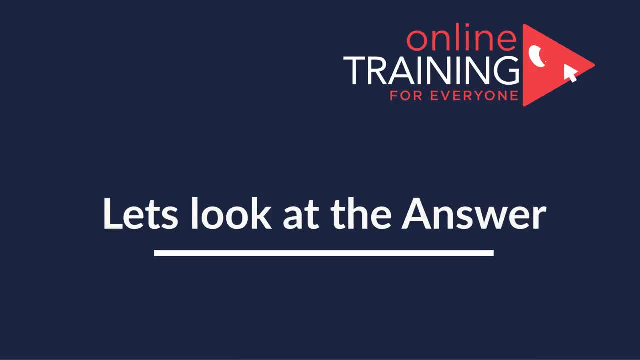 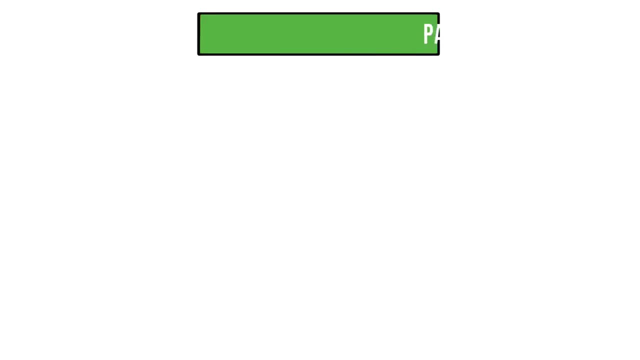 Did you figure out the solution? Let's continue to see how we can get to the correct solution together. The most important skill to solve this type of problem is the one that you can use to solve patterns recognition schemes. To recognize the pattern, you need to look closely into each column: Selective values. 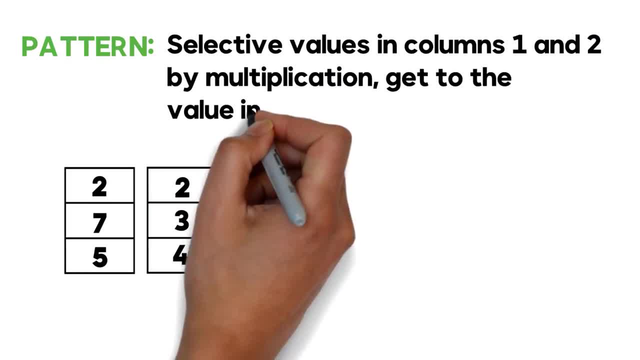 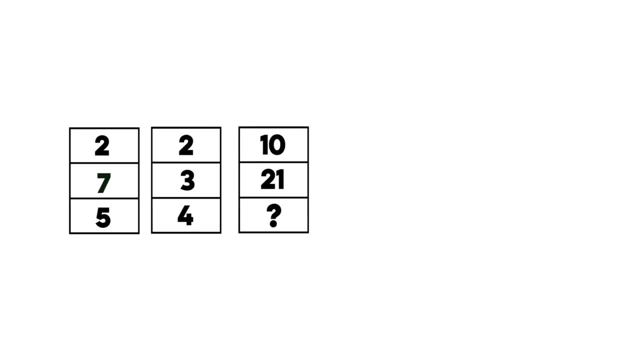 in columns 1 and 2 by multiplication get to the value in column 3.. And this is our pattern. Let's take a closer look for the values that are already present. If we multiply 5 by 2, we get to the value of 10.. Second set of values represented by the middle row: 7, multiplied. 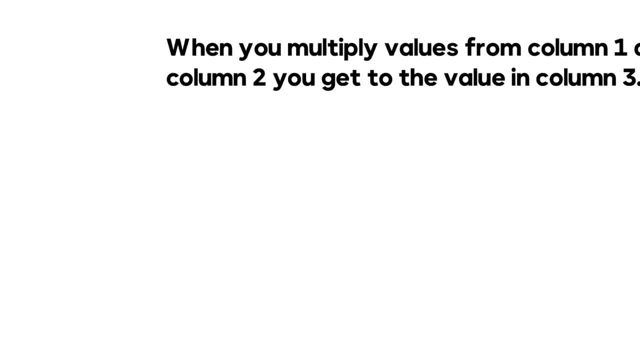 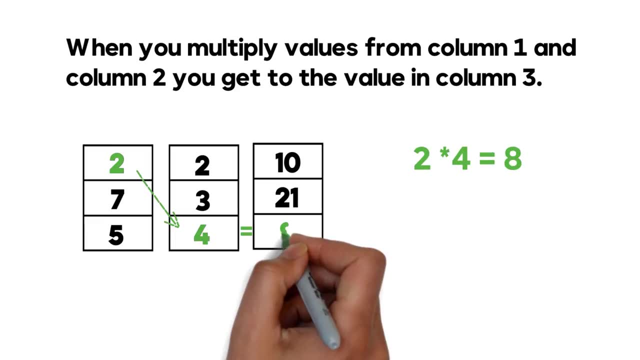 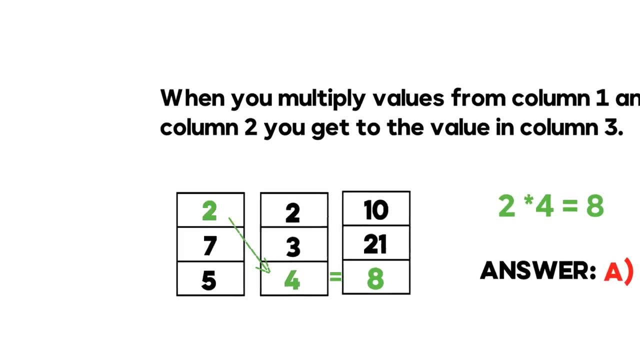 by 3 equals 21.. So the missing values here can be calculated by multiplying 2 by 4, and the end result would be equal to 8.. So the correct answer to this problem is choice A 8.. I also wanted to share with you one of the typical 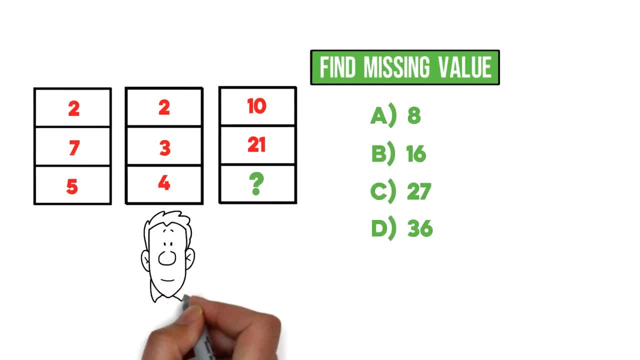 mistakes people make. as part of answering these types of questions, People start looking at the columns themselves, but unfortunately there's no pattern just by looking in the values in column 1, since pattern just doesn't exist If you look only at the values in column 1 or only at the values in column. 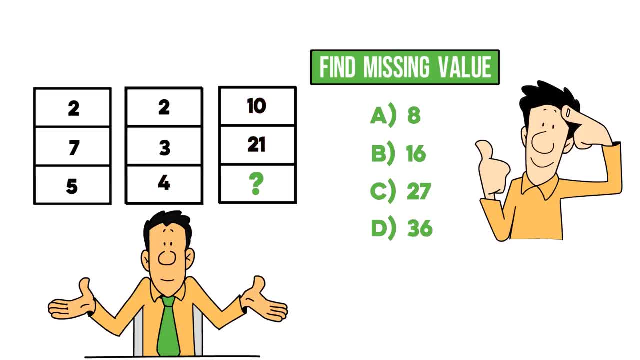 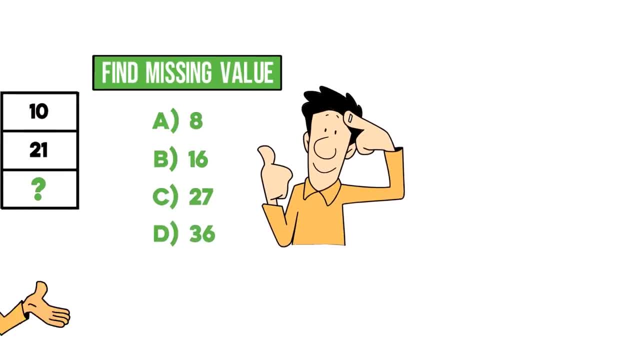 2 or only at the values in column 3, you will not be able to come up with the answer. You have to look across and take a global view across multiple columns to get to the correct solution. Can you do me a favor If you have a better way of? 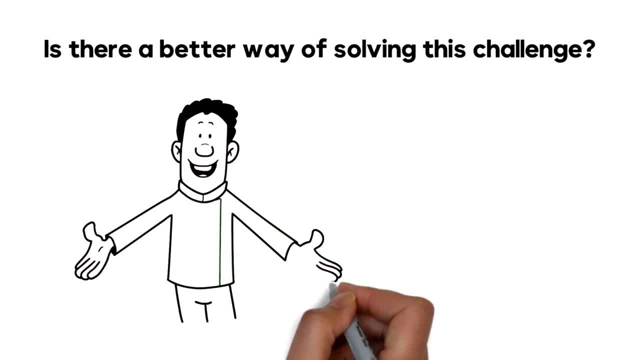 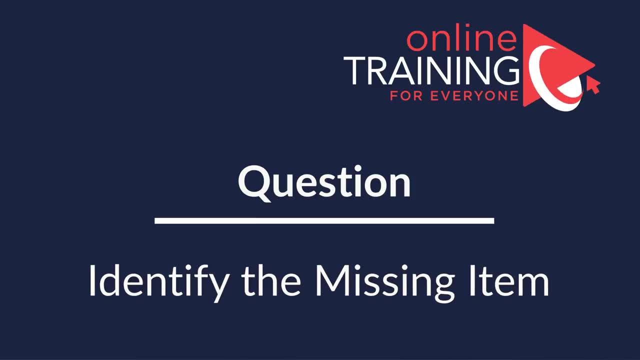 solving this challenge. please share your thought process in the comments section below. I'm excited to share with you a cool question which is easy to understand but which doesn't have an obvious answer. You're presented with the 2 by 3 matrix. 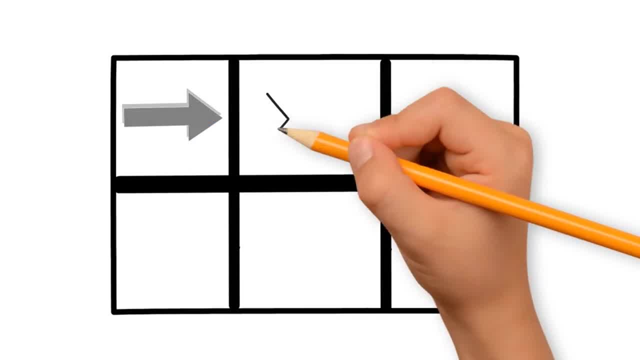 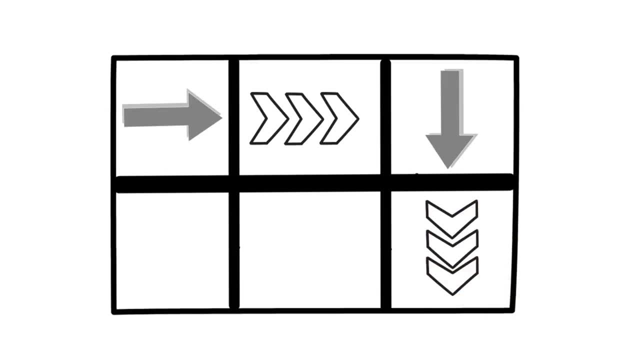 This matrix has arrows inside. There are two types of arrows: solid arrows, and then there are arrows that consist of three different shapes. There are six possible spaces in the 2 by 3 matrix. Five shapes are present and one shape is missing. 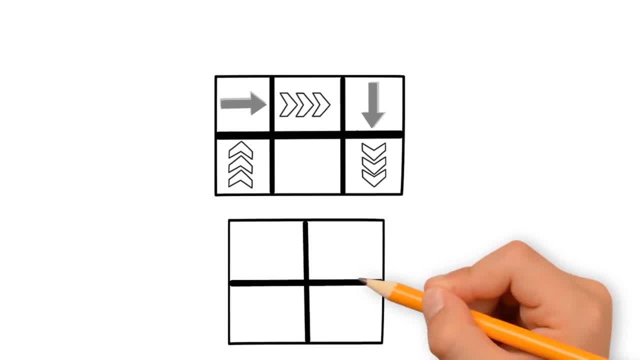 You're presented with four different choices to identify the missing shape which is highlighted by the question mark. You have choices A, B, C and D. Give yourself 10 to 15 seconds to see if you can identify the right answer. Did you figure out the correct answer? Let's continue to see if we can get to the correct. 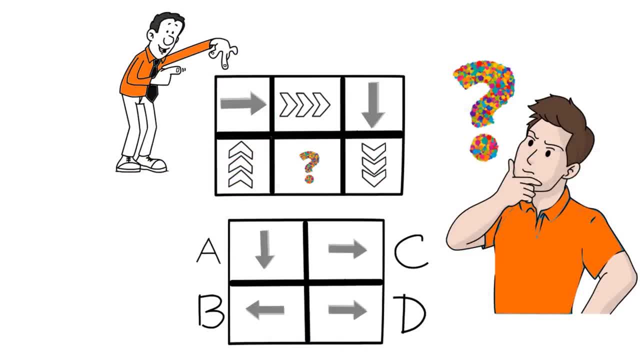 solution together. To solve these types of challenges, you always need to look for patterns, and there are three different patterns present in this sequence. Let's look at the pattern one. If we start from the upper left corner and go clockwise, you see that the arrows change. 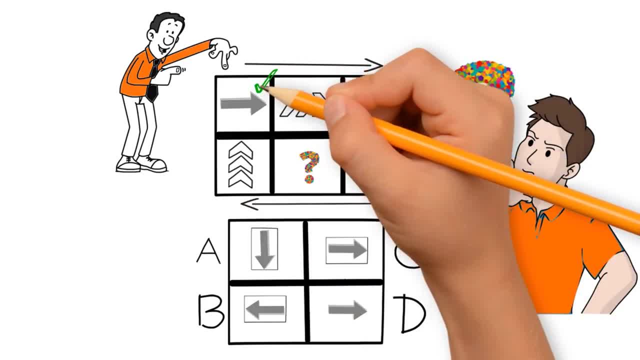 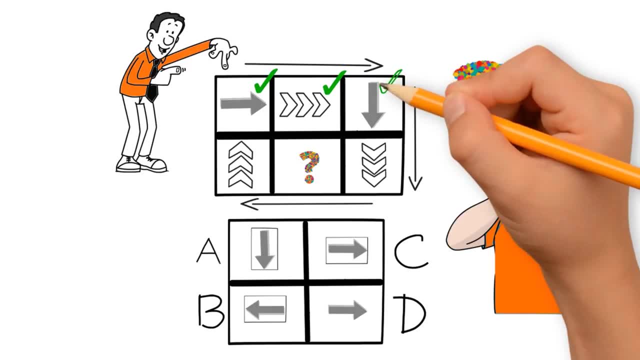 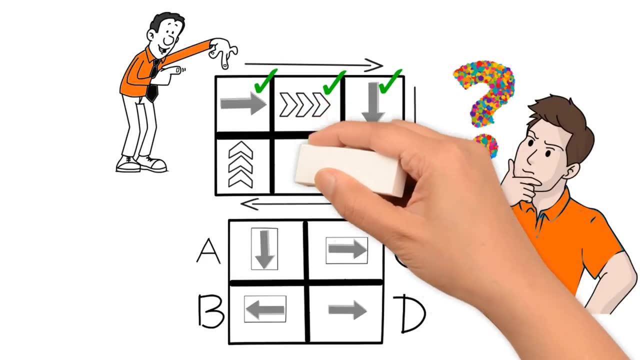 alternatively in each subsequent box. Second pattern is that inside the box, solid arrows rotate clockwise. and then the third pattern, which is a little harder to identify, is that the previous arrow points to the next arrow start. This is why the missing part, the part that you would need to identify, contains an arrow placed in the right corner. 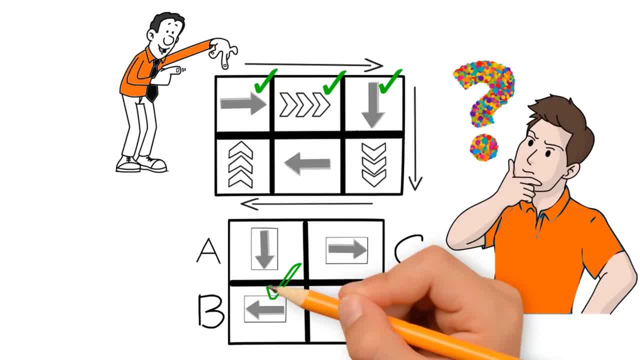 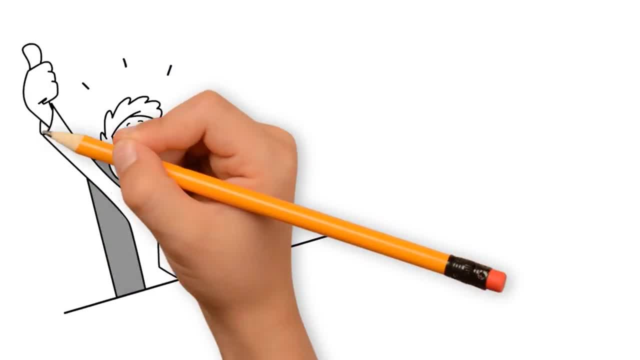 pointing to the left. So the correct answer here is choice B. Hopefully you've nailed this question and now know how to answer similar problems in the test. But in case you need more problems and solutions, please make sure to check out my ebook in the description section of this video. 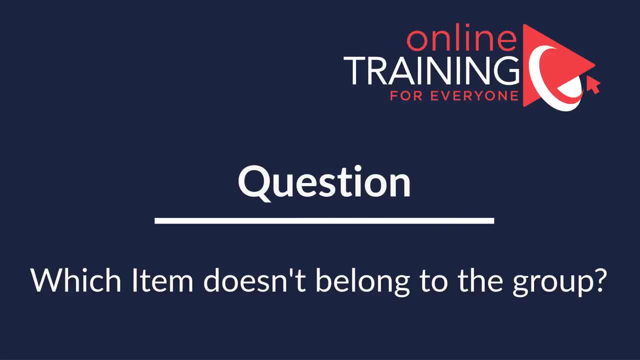 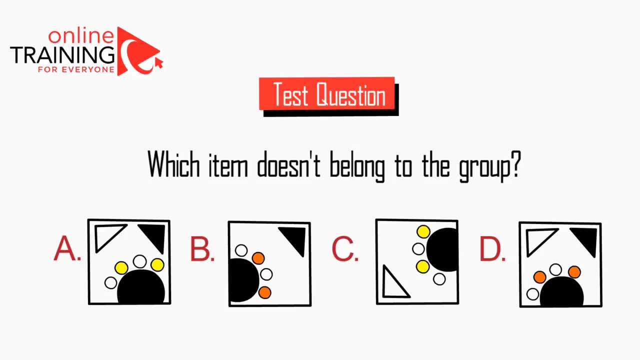 The types of questions you're looking at is very frequently used in the test. Typically, you're being asked to determine the item which does not belong to the group and you're presented with multiple items. In our choice, we have choices A, B, C and D. 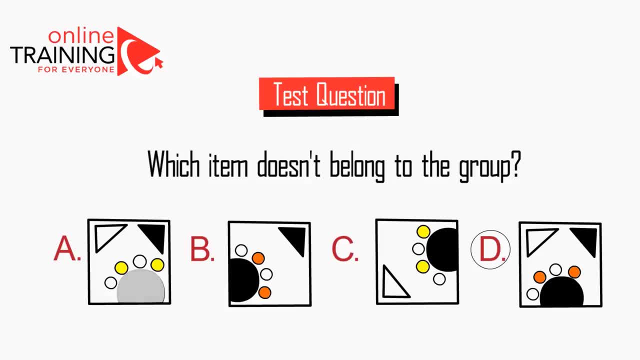 Each item is represented as a square which contains multiple different items inside, and you need to determine the item which does not belong to this particular pattern or sequence. Do you see the answer? Please take a look to see if you can come up with the solution. 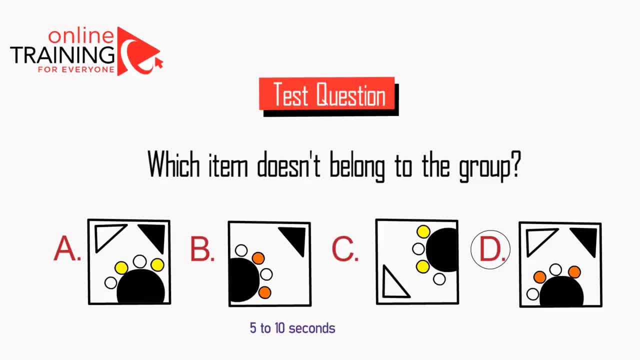 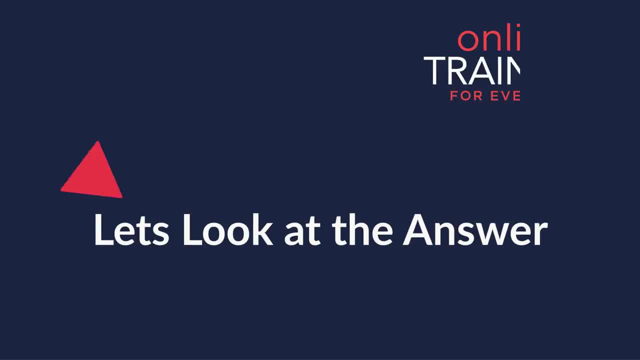 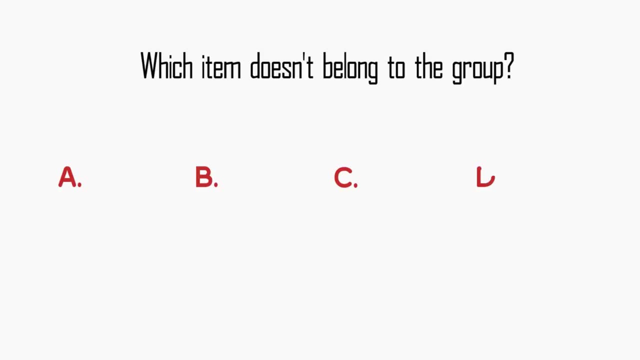 Give yourself 5 to 10 seconds, maybe 10 to 20 seconds, to see if you can come up with the answer. Did you figure it out? Let's continue to see how we can go and get to the correct solution together. As you might have figured out by now, there is always a pattern that you need to detect. 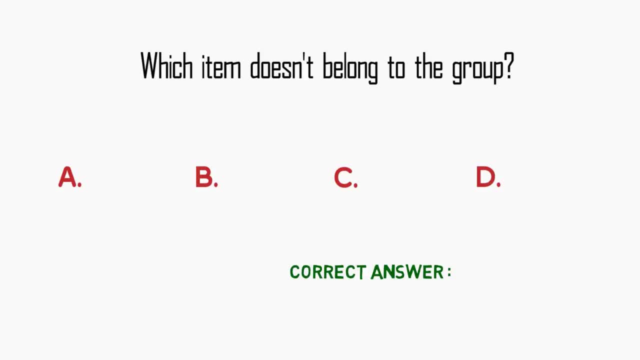 to answer these types of questions correctly, and a lot of times there are items that are designed to confuse you. So let me first walk you through the items that are designed to confuse you. You have small circles, and there are four small circles in each of the squares, and these small 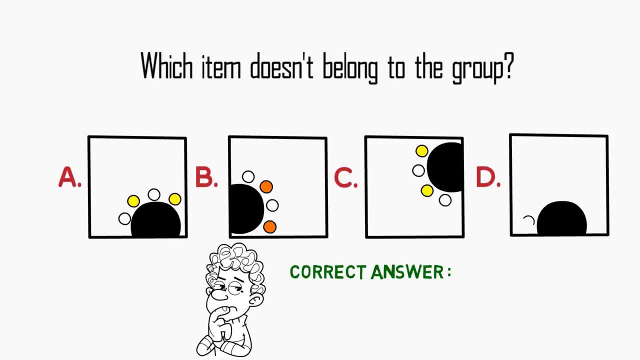 circles do not have any patterns. We also have triangles. Some squares have two triangles and some squares only have one. but there is no pattern here. The pattern is actually defined by the half circle and, as you can see, all half circles are attached to the corners of the square. You see this in the shapes A, B and C. 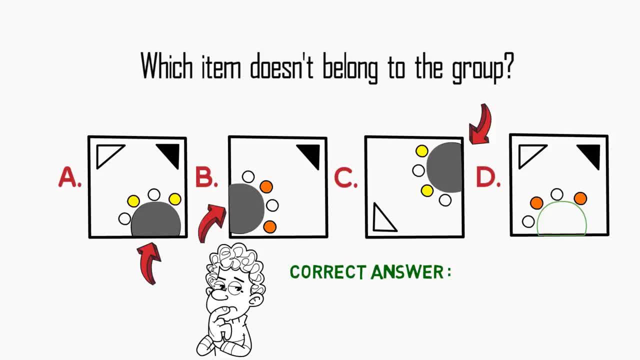 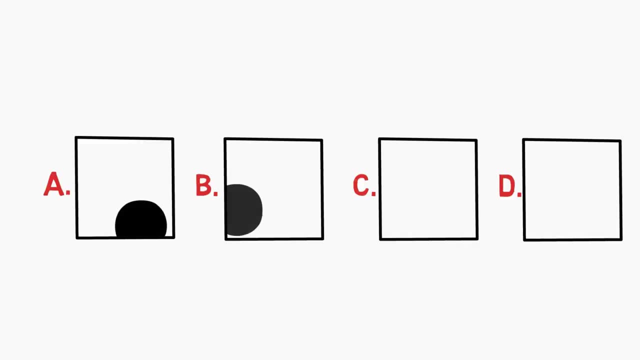 But in shape D half circle is placed in a different location. It is in the bottom middle of the square. This is why the item that doesn't belong to the group is the choice D. So the correct answer here is choice D. Let's recap: The pattern here is that all half circles. 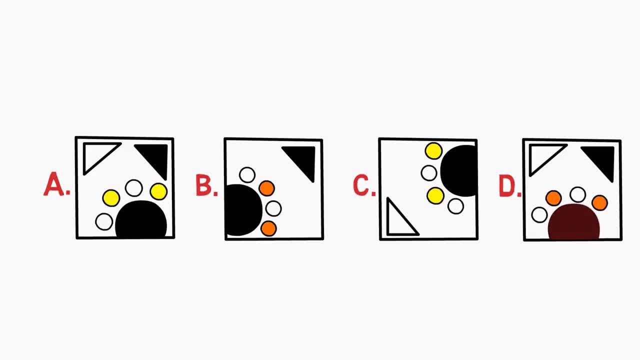 are attached to the corners of the square, but half circle in the shape D is placed in a different place than the others. The half circle there is in the lower part of the square. This is why the correct answer here is choice D. Hopefully you've nailed this question. 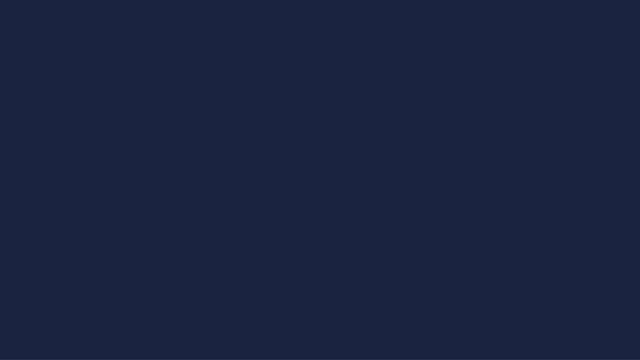 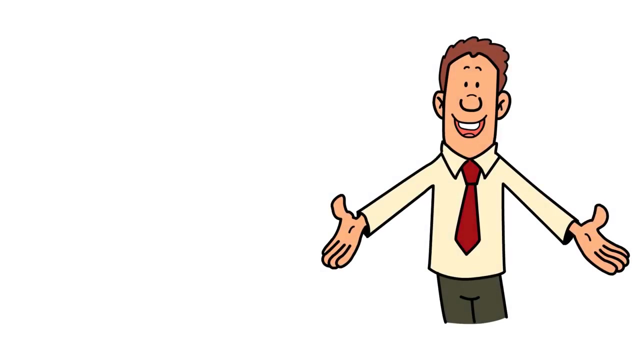 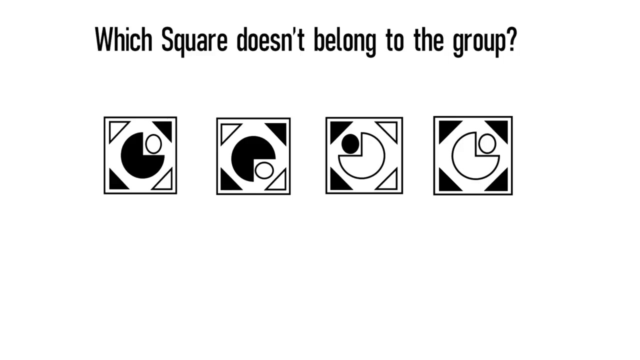 and now know how to answer similar problems on the test. I'm excited to take advantage of the opportunity and share with you how to solve these types of problems on the test. Typically, when you get a problem, you need to determine which object does not belong to the group. In this particular case, you need to determine which square doesn't. 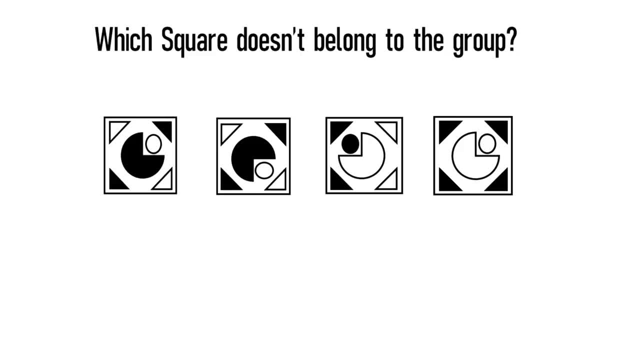 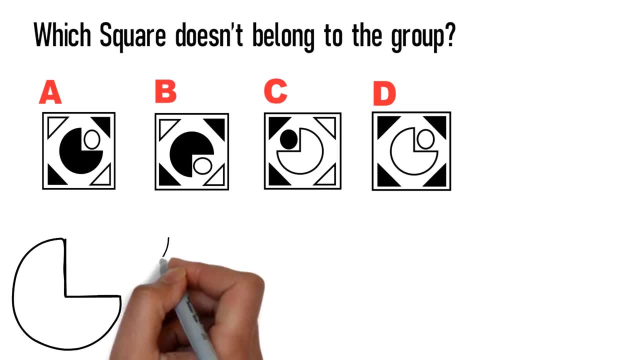 belong to the group. You're presented with four different squares, Choices A, B, C and D. Each square contains two circles inside. In the large circle, quarter of each circle is missing and instead replaced with the small circle. All squares also have triangles in the corner. 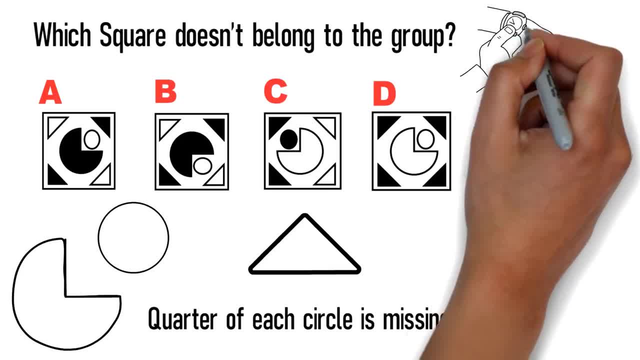 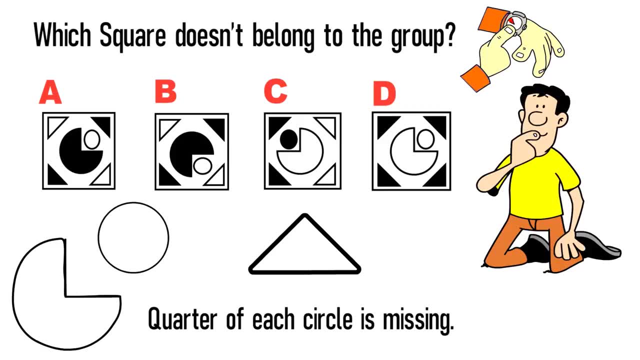 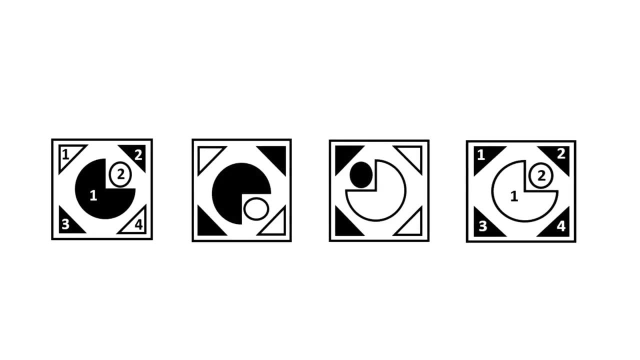 Give yourself five to ten seconds to see if you can come up with the answer. Do you see the answer? Let's continue to see how we can solve this challenge and get to the correct solution together. The key to solving this challenge is to detect the pattern. This is the skill that you need. 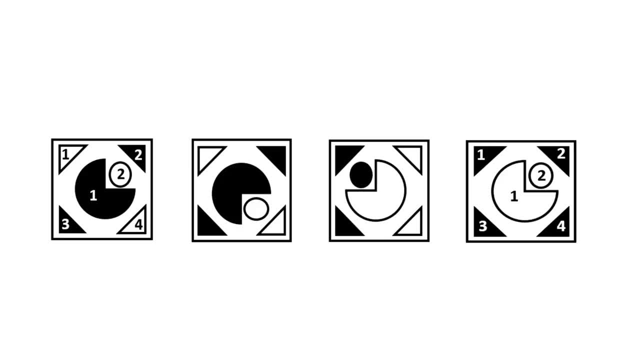 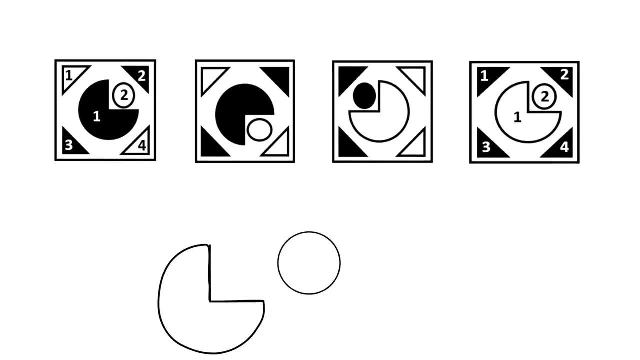 to develop to be successful in the test. Because there are two shapes here present in this question: triangles and circles. you should try to detect pattern among triangles and then among circles. In this particular question there is only one pattern Pattern of the triangles, But there are some sophisticated questions on a test which might include patterns for both shapes. 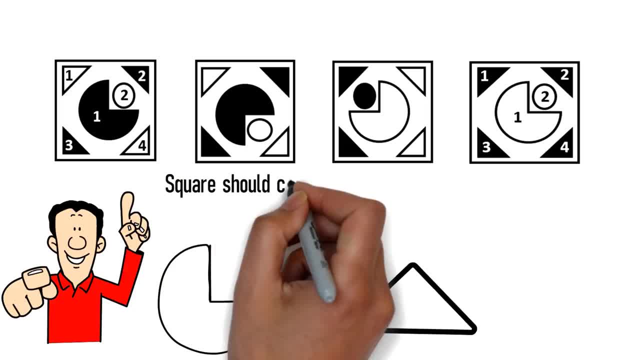 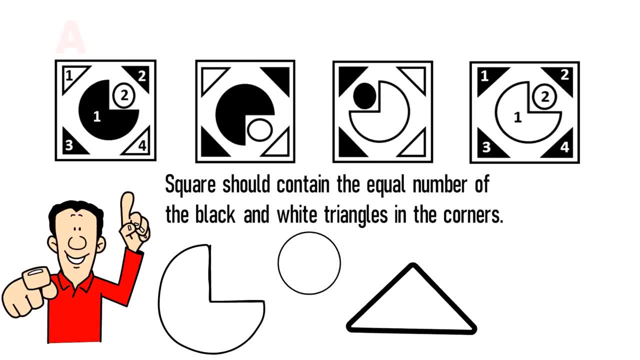 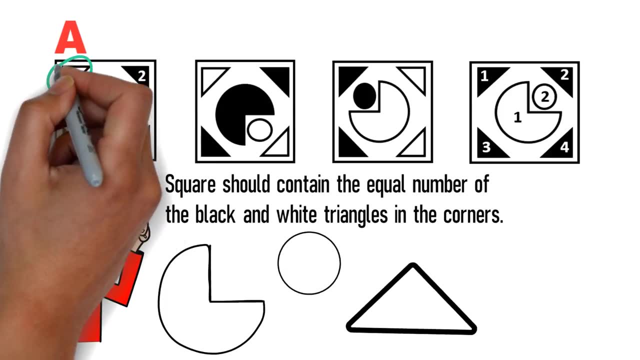 In this particular case, the pattern is that the square should contain the equal number of black and white triangles in the corners. Triangles in the square A positioned diagonally across each other. White triangles are located in the upper left corner and in the bottom right corner, And black triangles are located 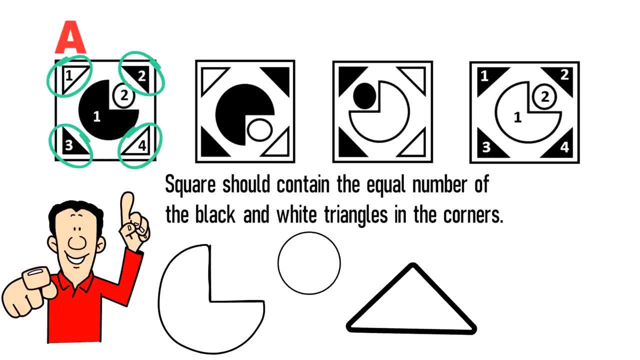 the bottom left corner and in the upper right corner. you can see that the same pattern exists in the shape b, two white triangles and then two black triangles, and in the shape c, two black triangles on the left and two white triangles on the right. but if we look at the choice d, 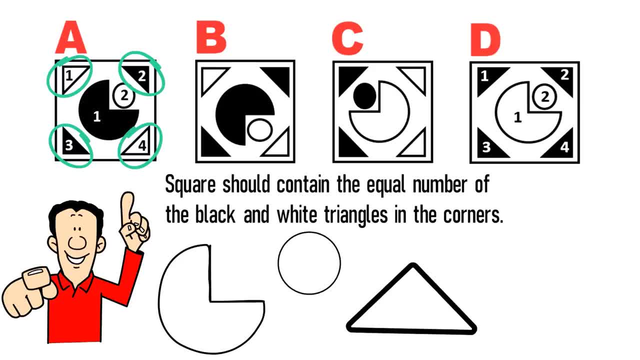 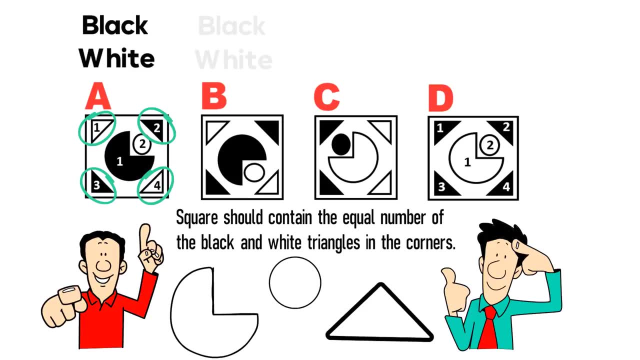 you see that there are four black triangles in the corners. circles in this picture do not have a pattern and their primary goal is to confuse you. if you look at the circles closely, you see that the large, small circle pattern doesn't exist. we have black white. shape b: black white. 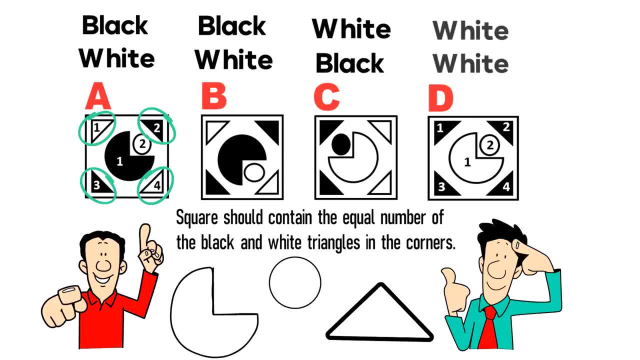 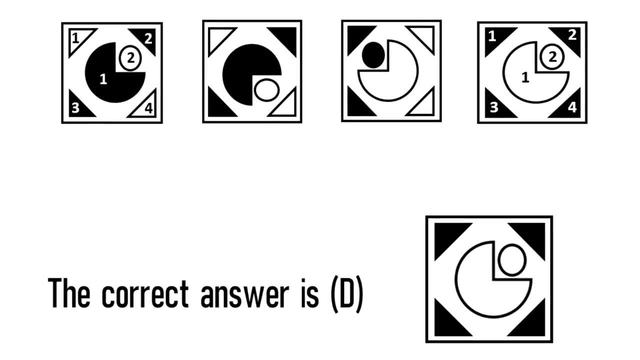 shape c- white- black and then shape d- white- white. based on this information about the circles, we should ignore them and focus on the triangles inside the squares. this is why the odd shape, the shape that doesn't belong to the group, is the one that does not have equal distributions of all colors in the corners. 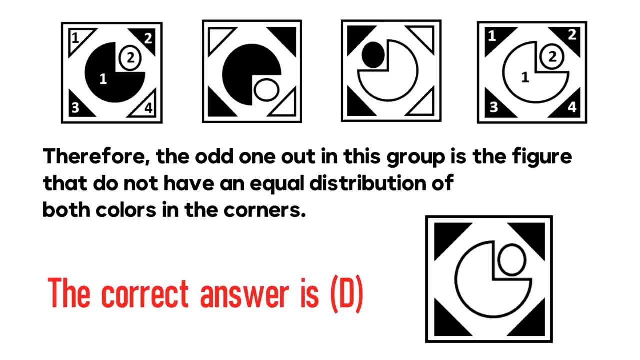 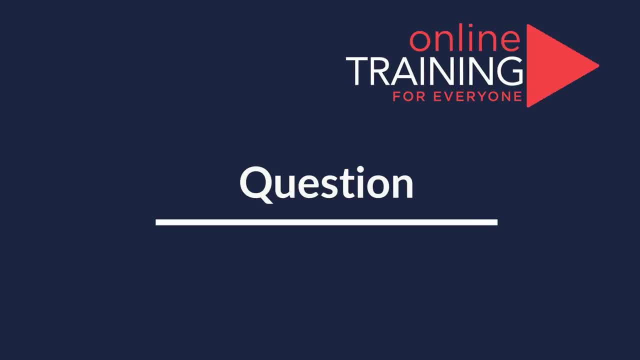 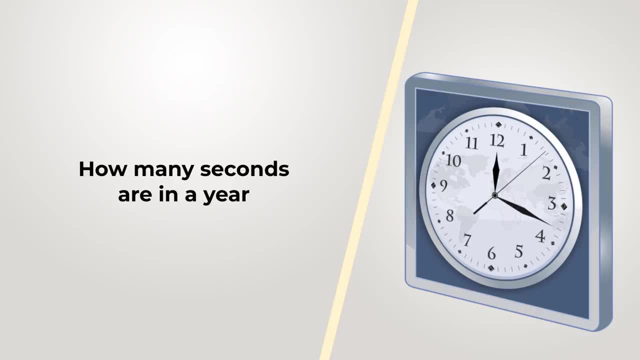 so the correct answer is yes. the answer here is choice d. hopefully you've nailed this question and now know how to answer similar problems on the test. i had this question being asked as part of consulting job interview. how many seconds are there in a year? take a look at the picture. it might give you a hint, do you? 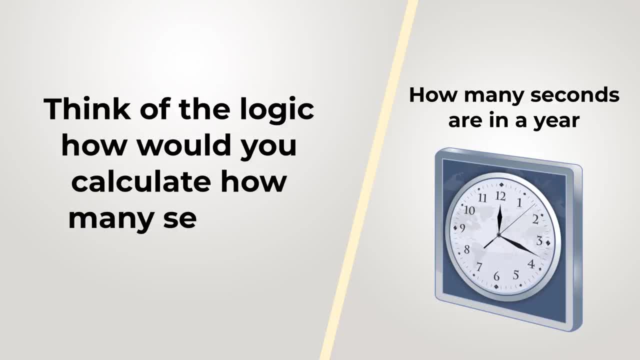 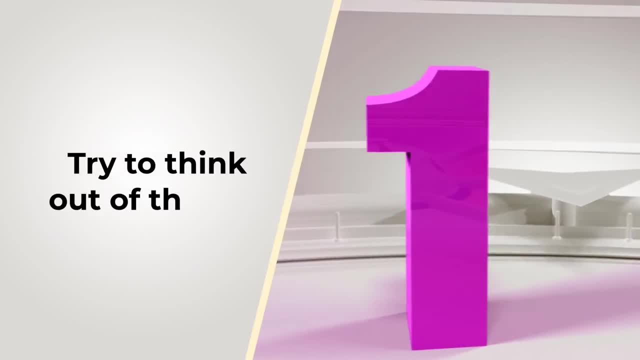 think you know the answer. think of the logic. how would you calculate how many seconds are there in the year? or maybe there is an alternative? always try to think out of the box- this would be my hint to you- and give yourself 10 to 15 seconds. this is as much time as you might get. 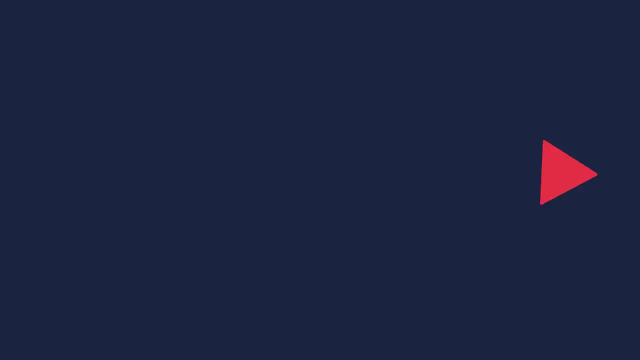 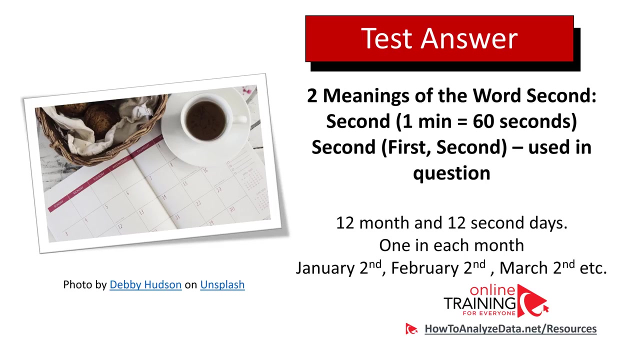 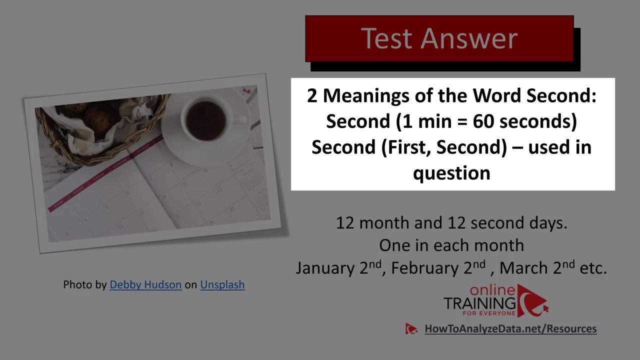 answering these types of questions in the test. now let's continue and get to the correct solution together. obviously this is a tricky question and it challenges you in understanding of the word second. there are two meanings in the word second. one is second- for example, one minute has 60 seconds- but second. one is second, where you 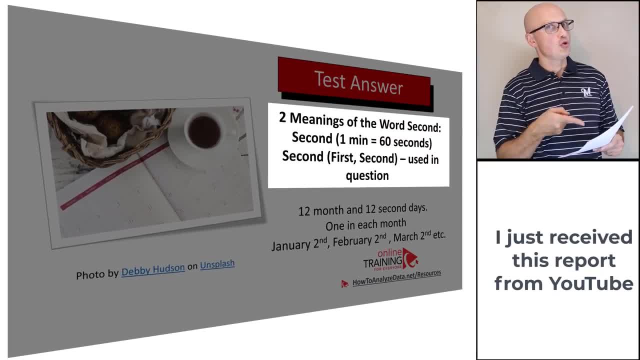 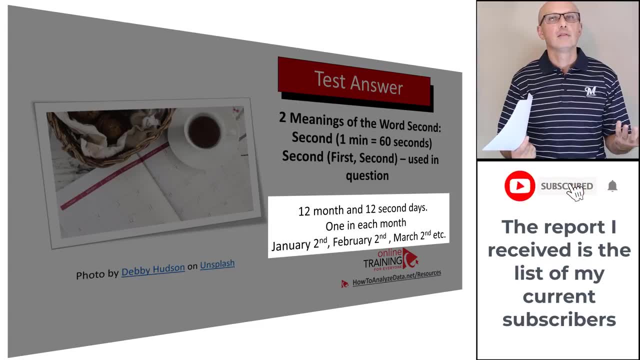 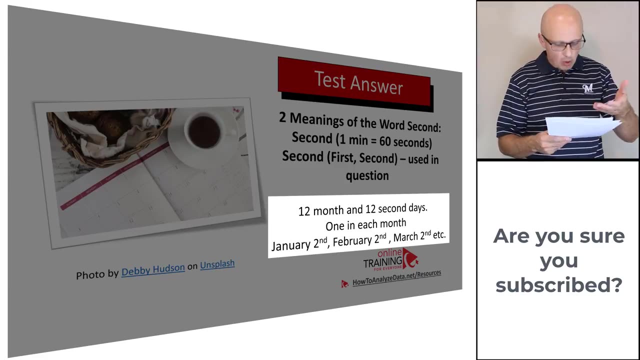 have a sequence of first and second and the second meaning of the second is used in this particular question. so if we go back to the question, in the year, there are 12 months and there are 12 second days, one second day in each month: january 2nd, february 2nd, march 2nd and etc. hopefully you've. 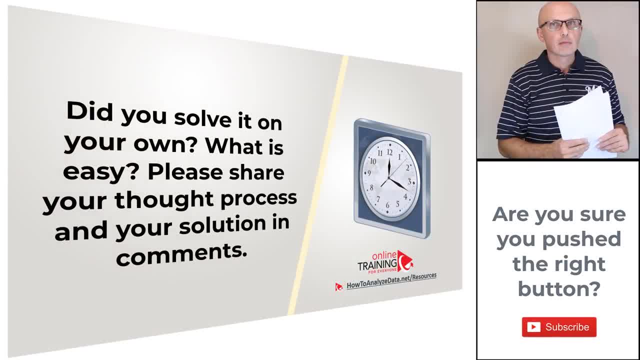 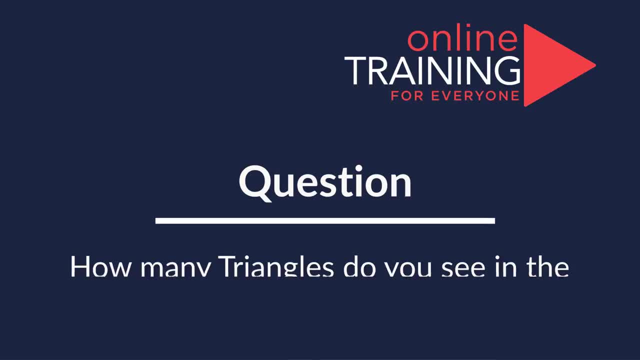 nailed this question. it gives you some laugh and you are able to answer this question in a few days. so until next time, bye, bye. You now know how to answer similar problems on the test. This is one of my favorite questions and there is a very high chance that you will get it on the assessment test. 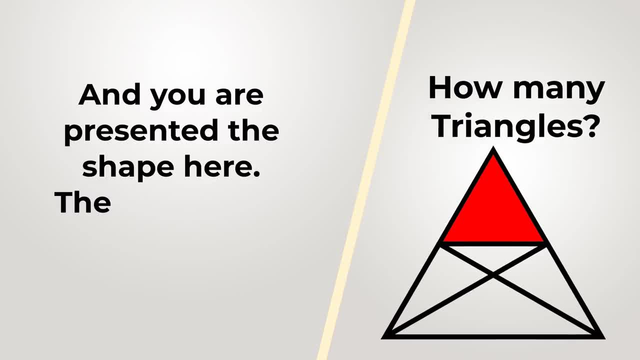 How many triangles do you see? You are presented with the shape on the left. There are large triangles and there are also lines inside of these large triangles. You have four different choices: Choice A – 9 triangles. Choice B – 12.. 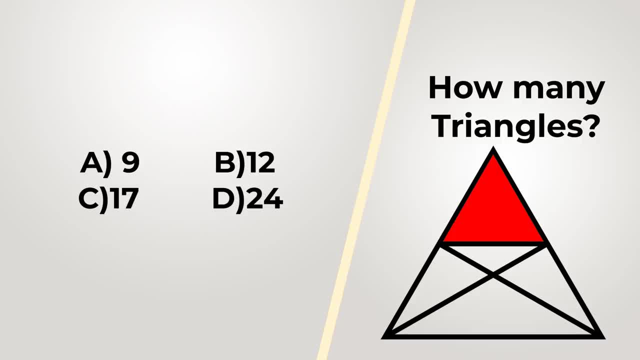 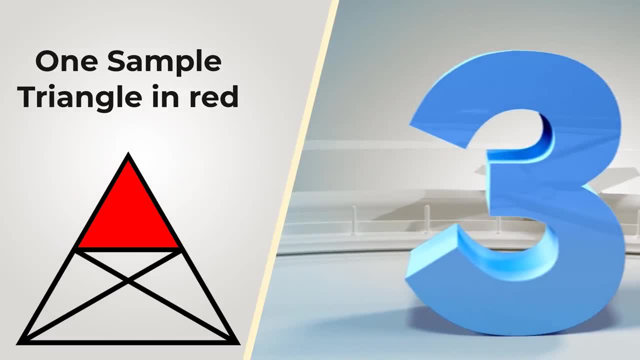 Choice C – 17. And choice D – 24.. One triangle is highlighted in red, but there are a lot of other triangles. Do you think you know the answer? Give yourself a few seconds. I would recommend 10 to 15 seconds. 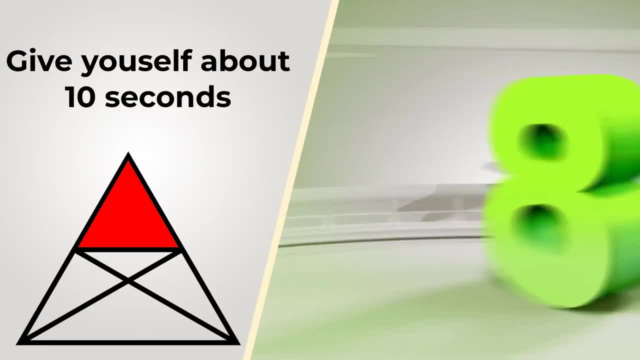 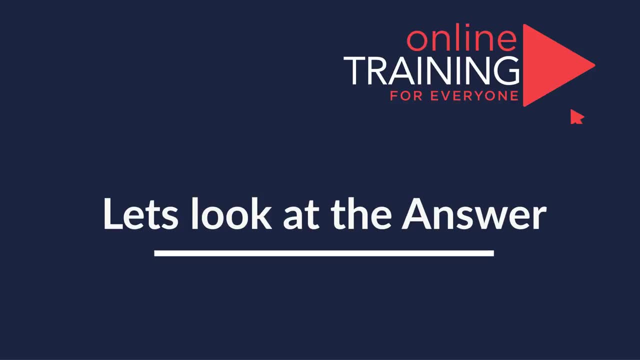 This is about as much time as you will get in the real test. You can pause this video to give yourself some time to figure out the answer. I am going to continue and reveal the correct solution so we can get to the answer together. I counted. 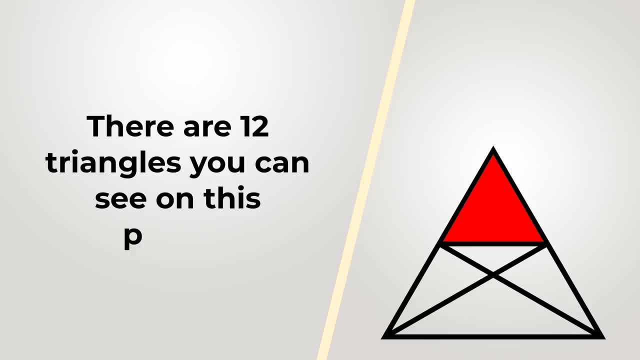 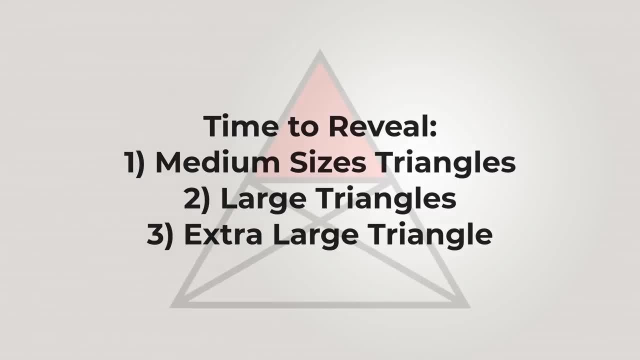 12 triangles on this picture. Is this what you got too? Let me show them all for you. I'll start with the smaller triangles and then go to the medium-sized ones and then go to the large ones. 1- 2. 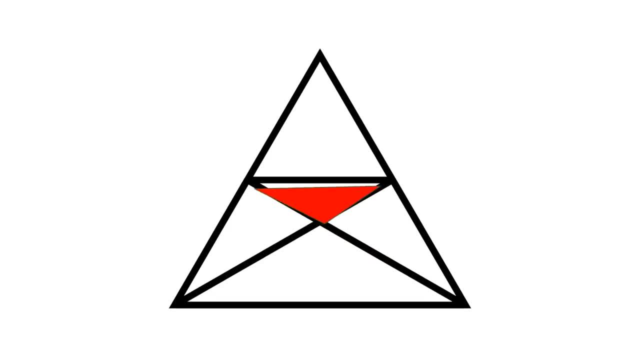 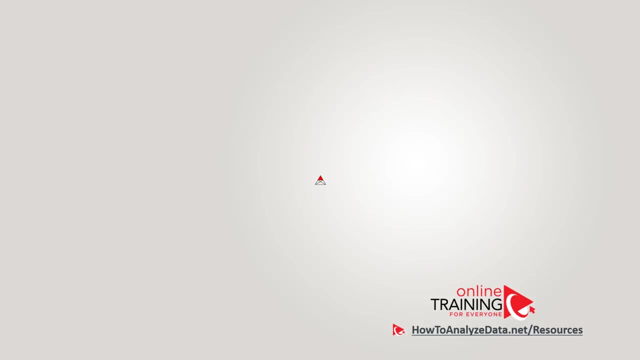 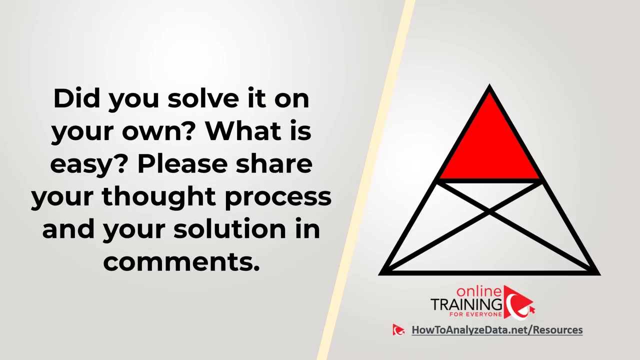 3, 4, 5, 6, 7, 8, 9, 10, 11, 11, 12. Did you come up with the different answer? Please share your thought process in the comment section of this video, so we can all learn from your perspective. 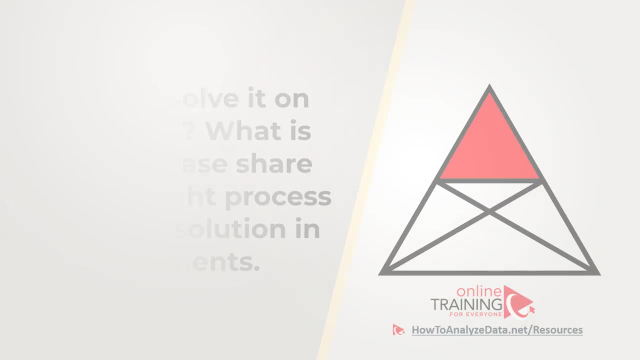 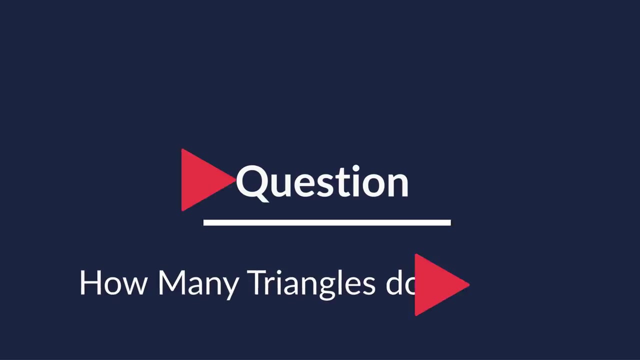 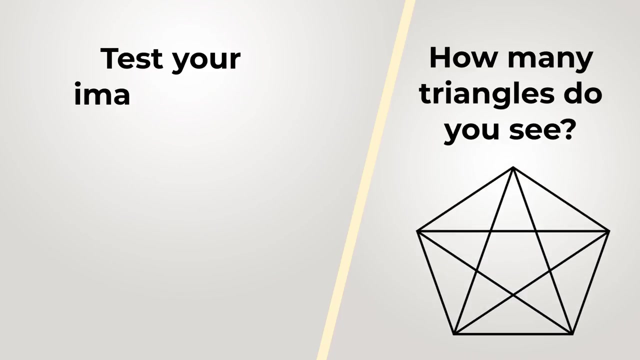 Hopefully you nailed this question and got to the correct answer on your own. Here is the very interesting question from the real test some of you might find challenging. Despite being tricky, you will have a lot of fun trying to find the solution Because this question tests your imagination. 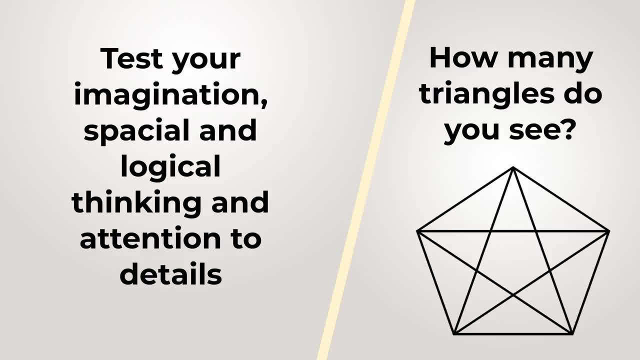 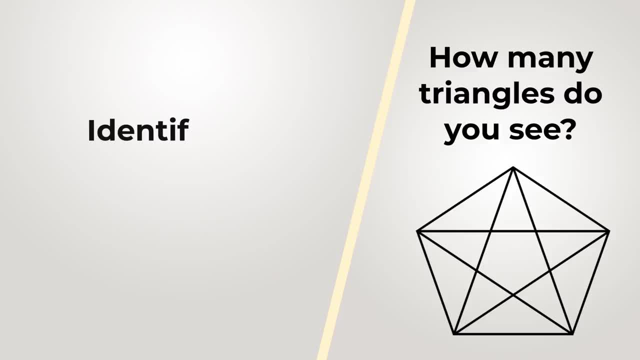 spatial thinking, logical thinking and attention to details. Now please take a look at the picture and identify all triangles on this picture. Do you think you know the answer? Now might be the right time to pause this video to see if you can come up with the answer on your own. 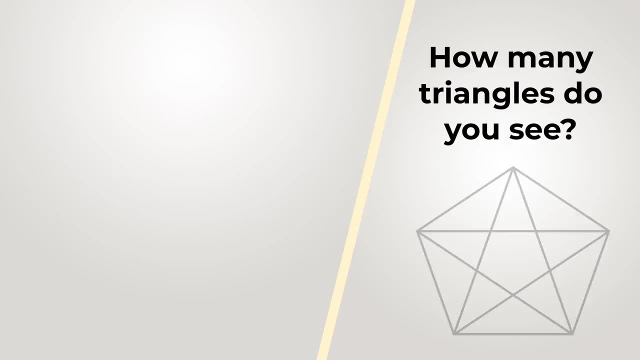 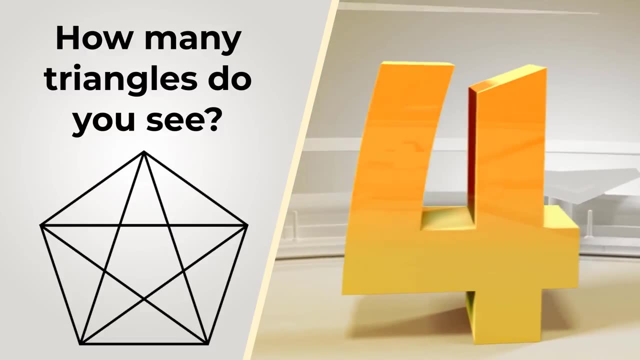 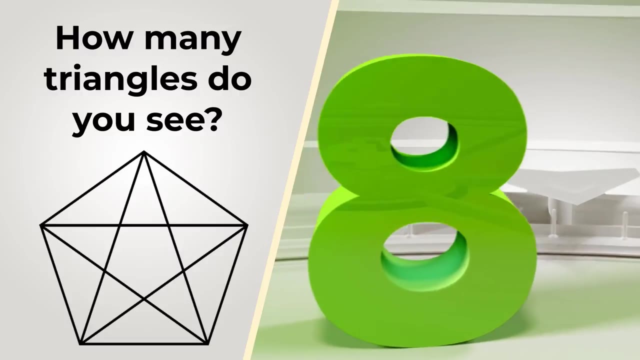 Give yourself about 10 seconds. This is typically about as much time you'll get on the real test. Did you come up with the answer? Let me give you a tip. Keep in mind, though, that in the real test, nobody is gonna give you any suggestions, But make sure to. 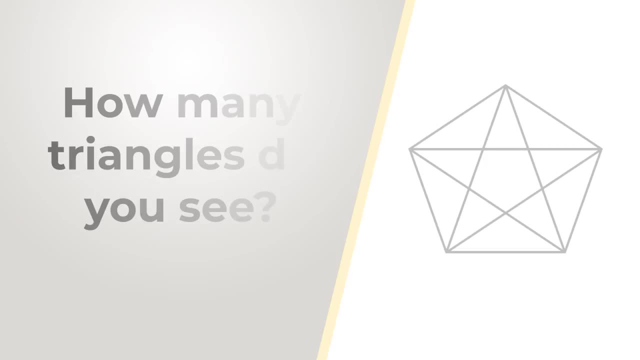 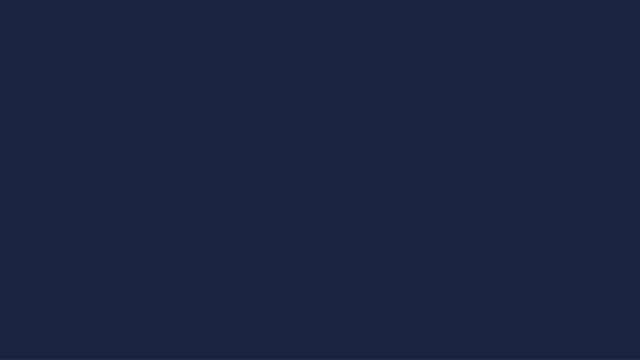 consider the possibility of one shape being inside the other. Now let's continue to see if we can solve this challenge and get to the correct solution together. It is mind-boggling, but there are 35 triangles here. Can you believe? it Certainly was a huge surprise to me as I was discovering them. Let me 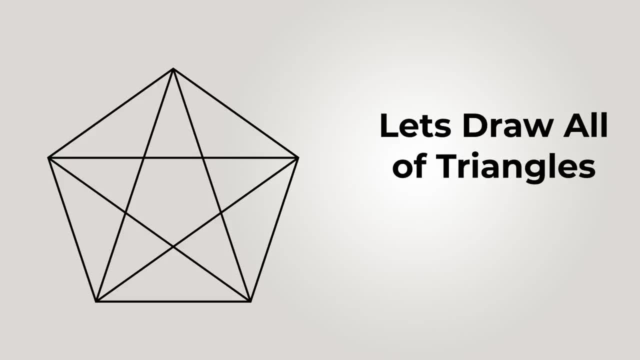 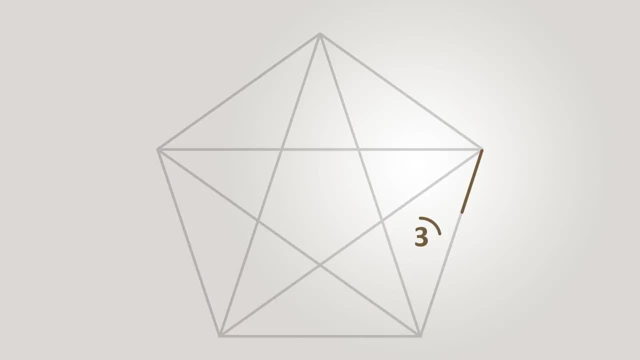 draw all of them for you. I will start by drawing small border triangles. There are 10 of them. Please count with me: 1, 2, 3, 4, 5, 6,, 7,, 8,, 9 and 10.. Now let's do next. 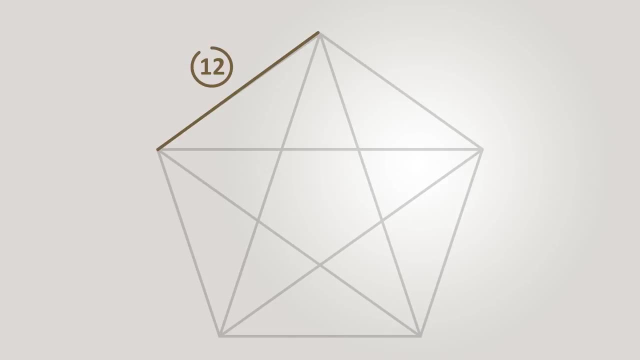 10 triangles: 11,, 12,, 13,, 14,, 15,, 16,, 17,, 18,, 19, And now let's do the next: 5.. 21,, 22,, 23,, 24,, 25. 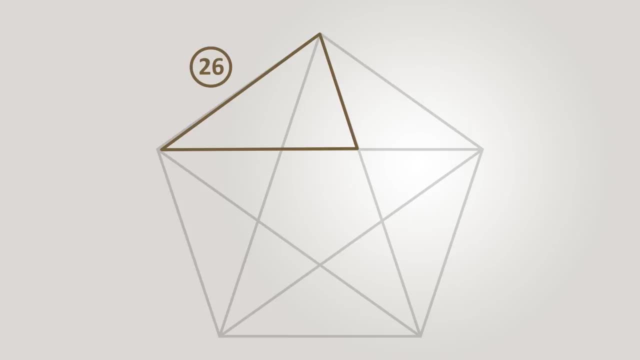 another 5.. 26,, 37,, 36,, 37,, 38, another 5.. 26,, 37,, 38,, 48, 27,, 28,, 29,, 30, and then the last five, 31,, 32,, 33,, 34, and the last one is 35.. 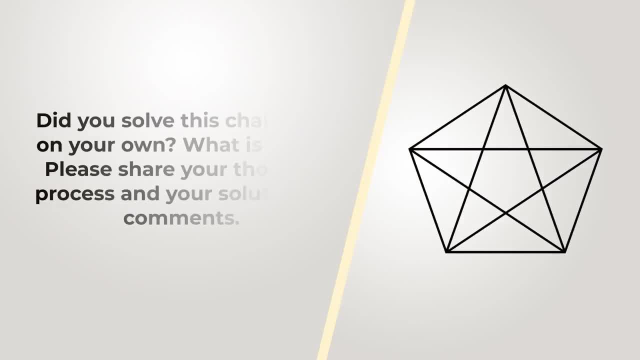 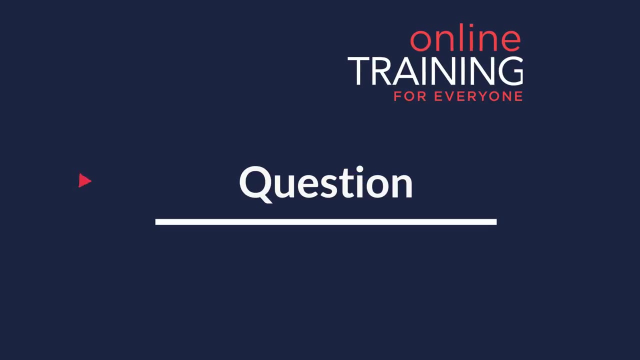 Do you think we missed any? Please make sure to leave your comment and let us know if there is even more. Hopefully you nailed this question and now learned how to answer similar questions on the test. Here's the interesting question you see sometimes on the test. It checks your. 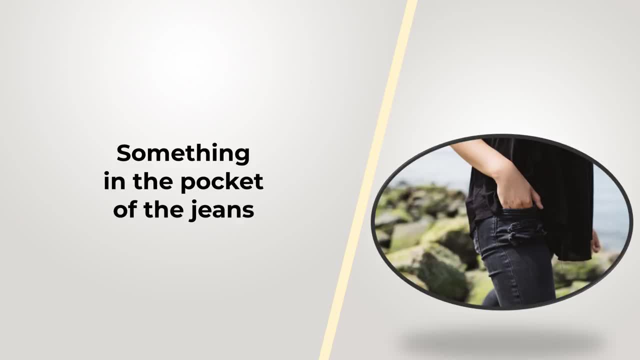 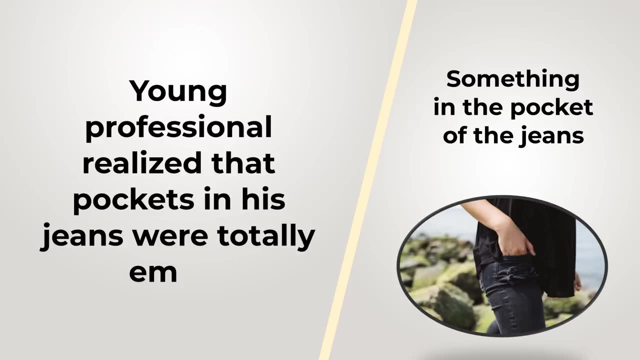 knowledge of verbal reasoning and understanding of the problem, And some people might argue that it tests your sense of humor as well. Young professional realized that pockets of his jeans were totally empty, But then he realized there was something else in there. How is it possible, Do you think you know? 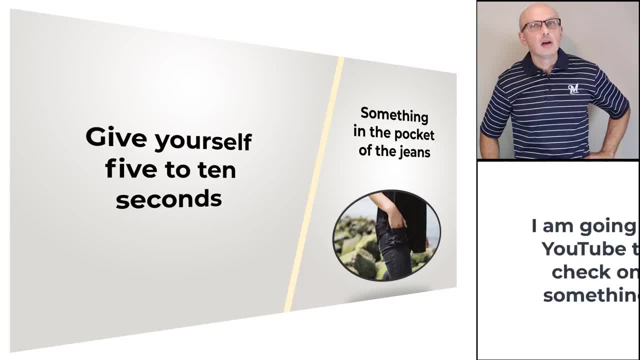 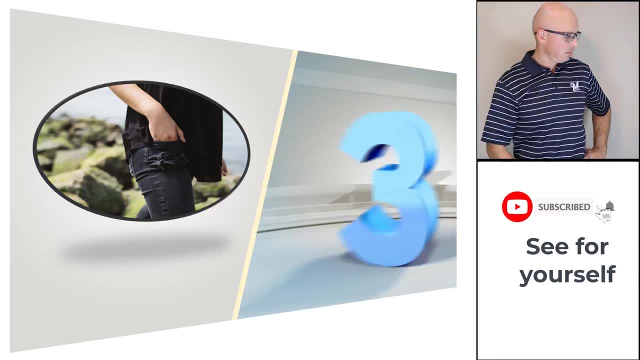 the answer? Give yourself 5 to 10 seconds, maybe 15 seconds. This is typically what you get on the test. Also, I'm gonna give you a hint. Please take a close look at the picture to see if you might see something unusual. Do you think you know the answer? Let's continue to see how we can solve. 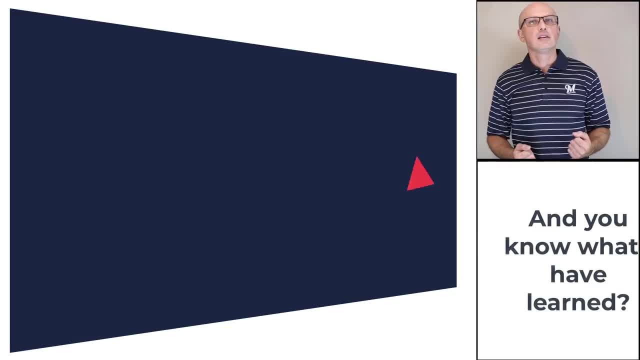 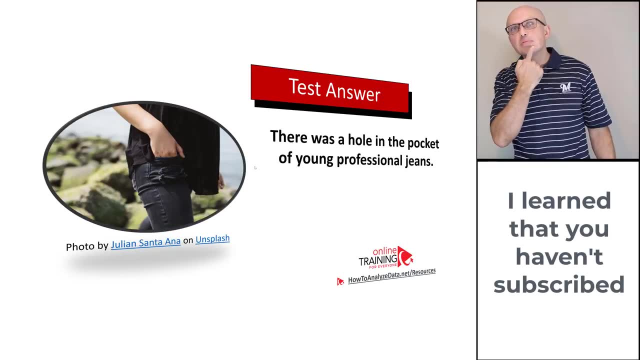 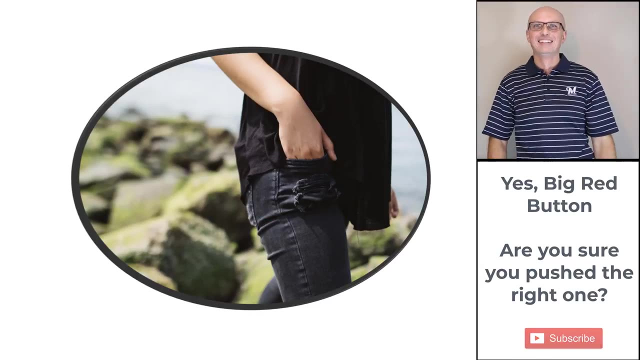 this challenge and get to the correct solution together. And the solution is very simple: There was a hole in the pocket of the young professional's jeans. Hopefully you've nailed this question and now know how to answer similar problems on the test. Thanks for watching. If you liked the content, please give us a like and consider subscribing.